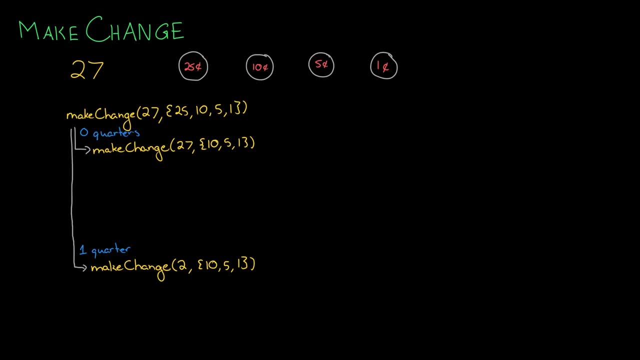 then we're trying to just make two cents from the remaining options, which obviously there aren't a whole lot of ways of doing that Now we just repeat this process. So how many ways are there of making change, of making 27 cents? 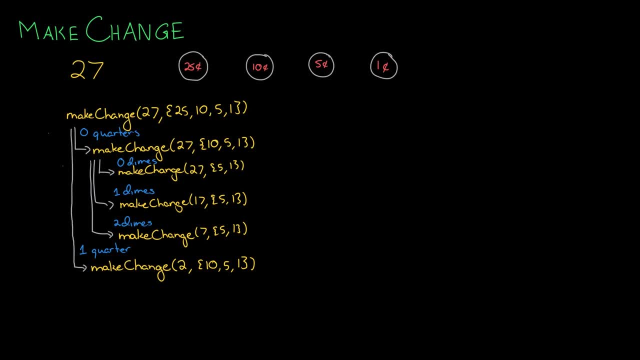 from dimes, nickels and pennies. Well, let's go through the different options. We could give zero dimes. Let's start with dimes, Zero dimes, one dime or two dimes And same thing for this other one, but the possibilities are much more limited there. 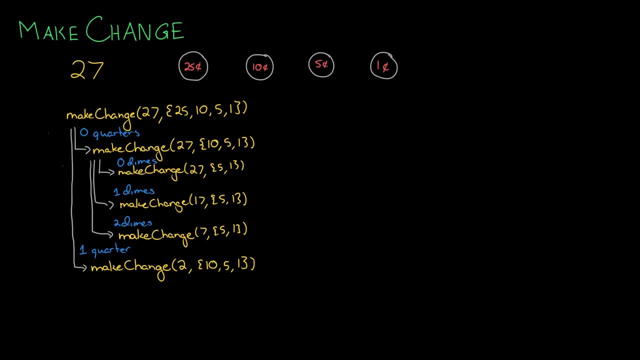 So if we keep going through this process, we'll eventually get to the point where we have a definitive answer. So if we're saying, how many ways are there of making change from 17 cents, given just pennies, that's one. If we're saying, how many ways can we make change of 17 cents? 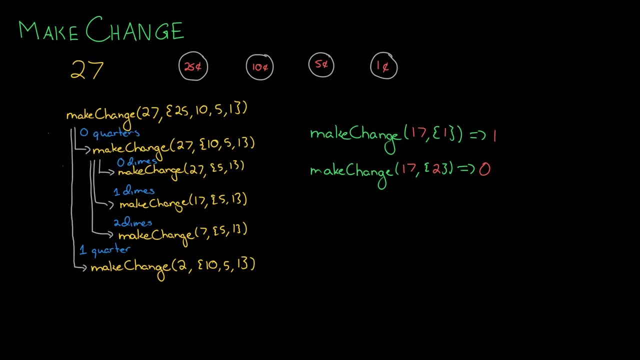 from just a two cent piece. so this is with different denominations. that's gonna be zero and those will be our base cases. So let's try a new example here with a bigger value and a little bit more denominations. So suppose we're trying to make 79 cents from half dollars, quarters, dimes, nickels and pennies. 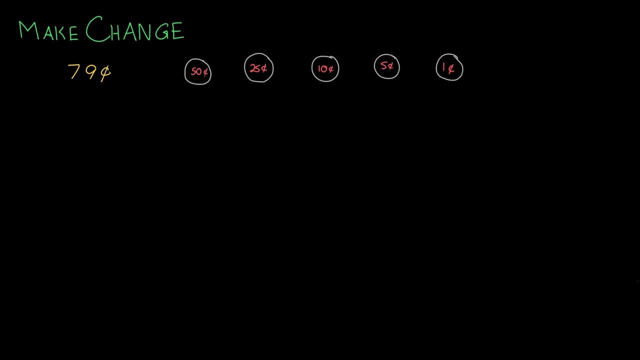 So one option we'll explore is making 79 cents with zero, half dollars and two quarters, and then the remaining 29 cents from dimes, nickels and pennies, pennies. Another option, though, that we'll explore is making 79 cents from one. 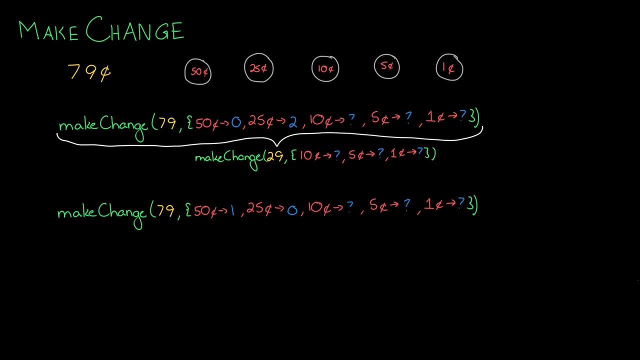 half dollar and zero quarters and the remaining 29 cents from dimes, nickels and pennies. So note that these two problems have now these two paths have reduced to the same sub problem. So, although we got to them in a different, 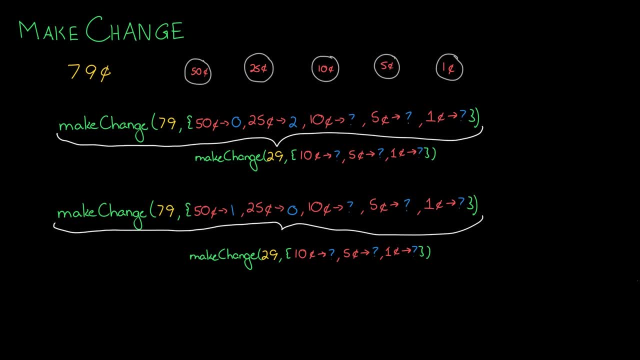 way one uses 50 cents, a 50 cent piece, and the other one uses two quarters. they have the same sub problem. So we don't need to compute this twice. Once we've computed it once, just store it for future problems. So that said, let's turn. 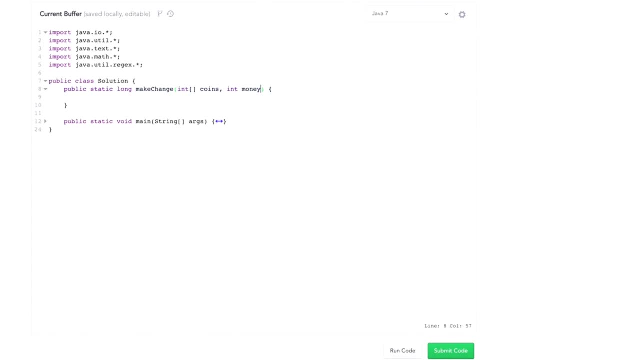 to the code. now, Whenever I do a memoization problem, I like to start off with just a straightforward recursive approach, because it helps me wrap my head around the problem a little bit better. So this is a make change function and it's just going to be straightforward recursion. It's going to return a long 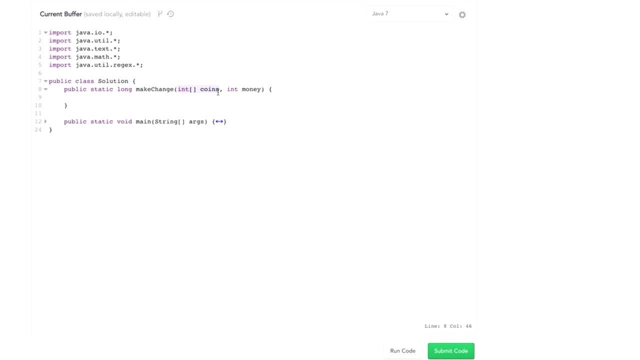 so that I can avoid integer overflow, and it's going to take in the denominations and the amount of money. Now, when we just talked through the problem earlier, we had had this array basically popping off the table and it was going to take in the amount of money. So I'm going to 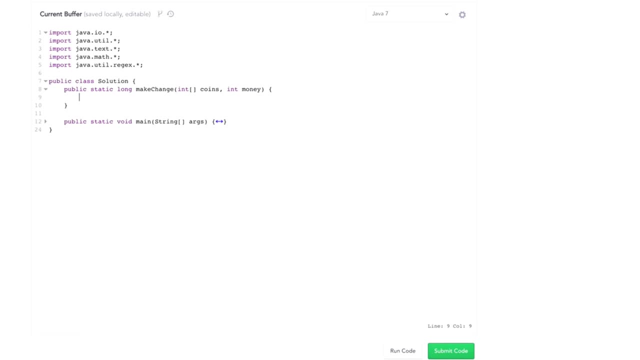 stop the first element That can get kind of inefficient to shift and shrink this array because that actually requires creating a new array. So a better approach is to just pass in some sort of index which tells us what coin we're currently considering. So we're going to do is take, you know, take the first coin. 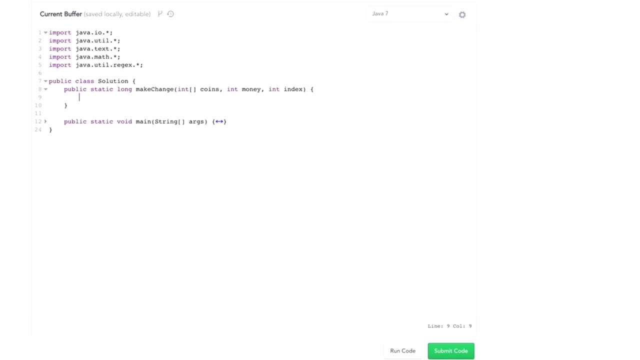 or take whatever index is pointing to, and if it's say 25 cents, consider saying: what if we have one of those or zero of those, one of those, two of those, etc. And I'm going to come back and add the base cases later. 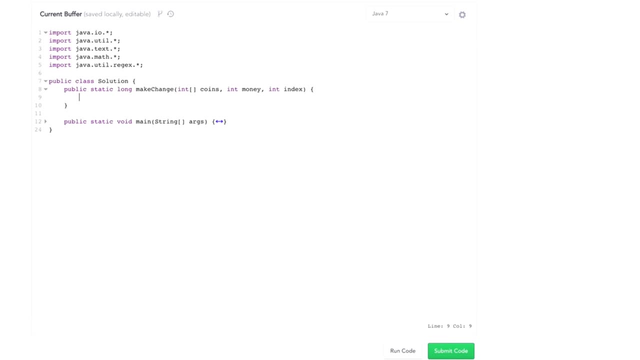 So the what I'm going to do is recurse on each of these options. So this is going to be the amount of money we have used from this particular coin. So while amount with coin is less than or equal to the amount of money, then we're going to say, okay, the 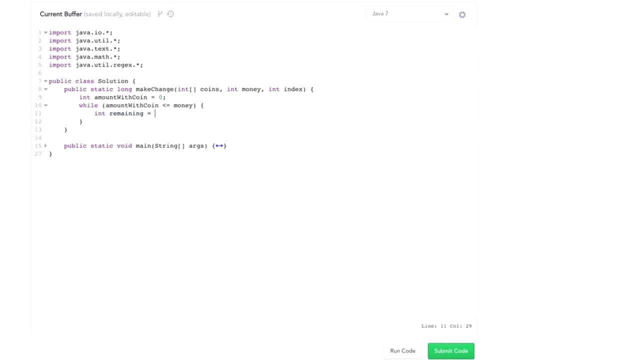 amount of money remaining we need to make is coins of index money. It's money minus uh amount with coin, Then recurse on this. So I'm going to need some long number of ways, Recurse on this and add that and keep track of that sum as we go Remaining. 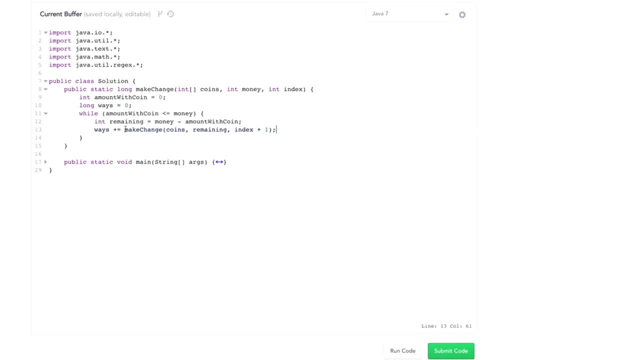 index plus one. So count how many ways there are of making the remaining amount of money with the remaining coins And then increment amount with coin By the value of that coin. We could alternatively actually just have amount to go from zero, one, two, three, four, and then multiply that by the size of the coin. Doesn't really matter. 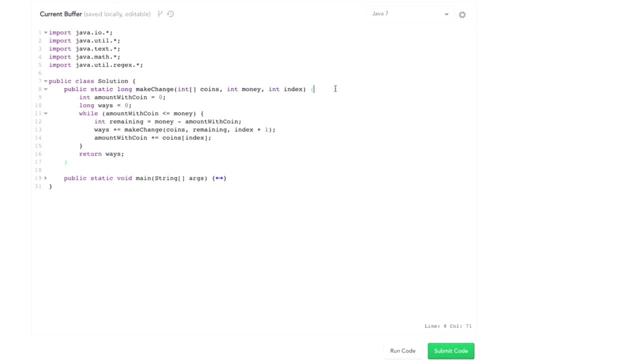 too much, which approach we make And then return ways. Now my base case is here: Well, if we're out of money, then so if we have zero, zero cents left, then well, how many ways are there making zero cents? 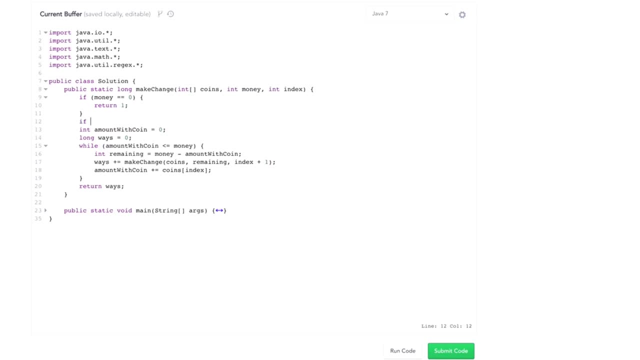 If it doesn't really matter what the coins is, then one. If we've run out of coins but not money, then the options are zero. So if index is greater than or equal to coins dot length, then return zero. So that's our recursion. It's always nice to give the caller a little. 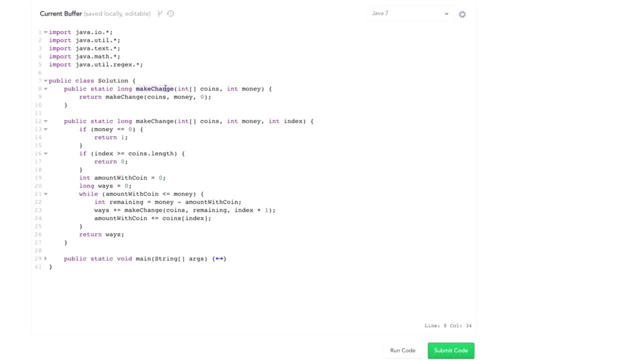 helper function. just to wrap that, because it makes it a little bit easier, So they don't have to worry about the parameters are Okay, now the memoization part. The idea here is that whenever we start to try to recompute the same problem and we want to say 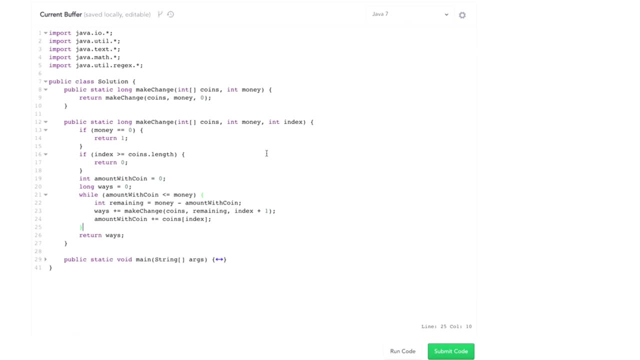 wait, we've already done this before return this stored value. The question is, how do we define whether or not we've seen the problem before? Sometimes people will use just money. We'll use some sort of hash map right that maps from the problem. however, we represent it to the number. 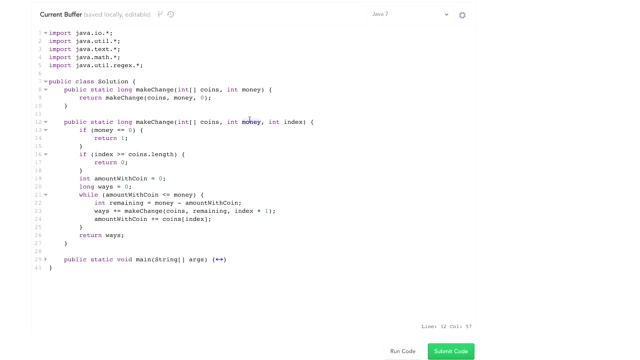 to the answer to that problem. So sometimes people will use money as the key in this hash table and that's actually not sufficient. Just because we're trying to compute the number by making change from 29 cents doesn't mean the number- the coins being used there are the same. 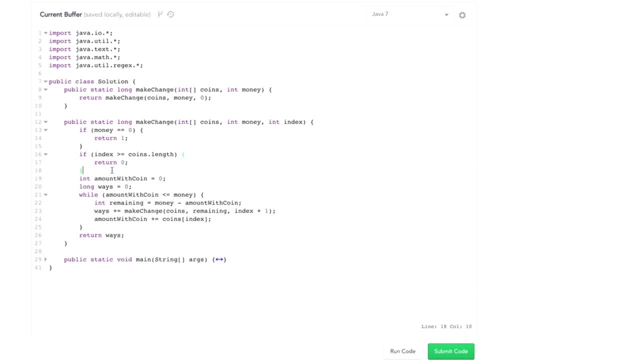 So we need a key that actually represents both the money and the index, So we could use a class that wraps both of those. but even simpler is a simple string. So just use a simple string. that's basic concatenation of money and index, And then we'll have a memo table that I'll use. that'll be a 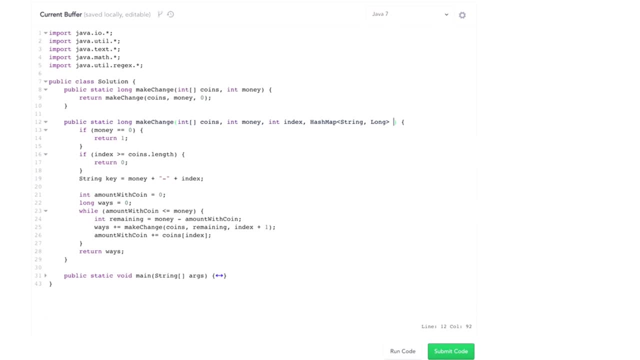 hash map, that maps from a string to a long and I'll call that memo. And now I'll say: if memo dot contains key of key, return memo dot get of key. and then at the very end here update my memo table of key comma ways. And when I call this function, 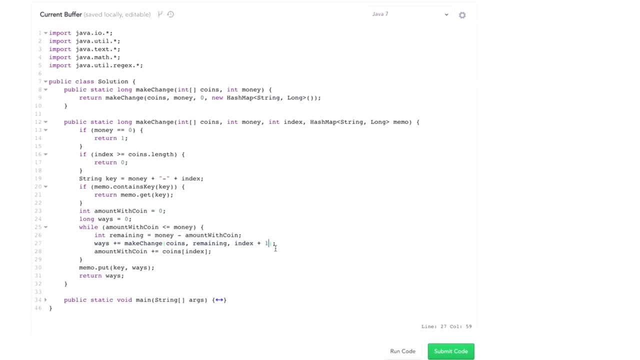 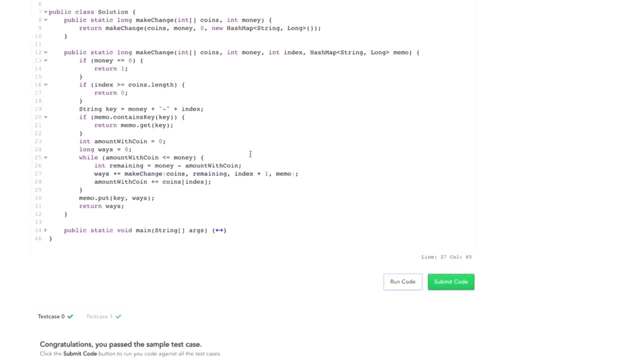 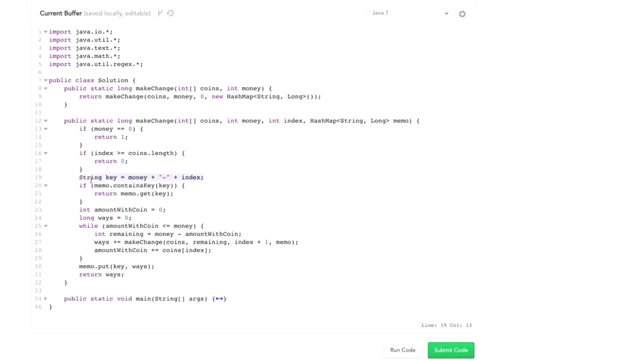 I'll pass in that memo table And then I also need to pass it in down here, Okay, So hopefully this will work All right. So now one thing I want to point out here that is a very common mistake for candidates to make: is this key? So here I've concatenated. 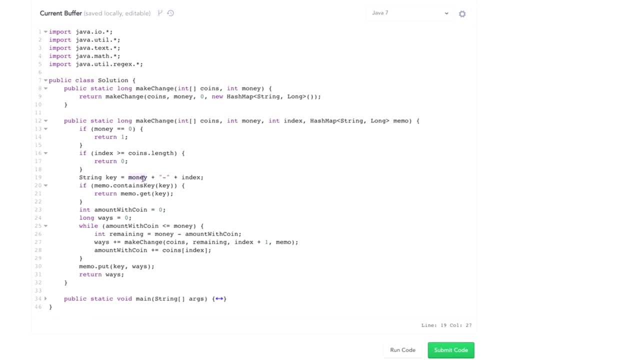 basically created a string representation for the money and the index. You want to make sure there's a separator there, because otherwise you could have a situation where you're concatenated, like you know, let's say 29 plus one, and that gets confused with two plus 91. So just be careful.